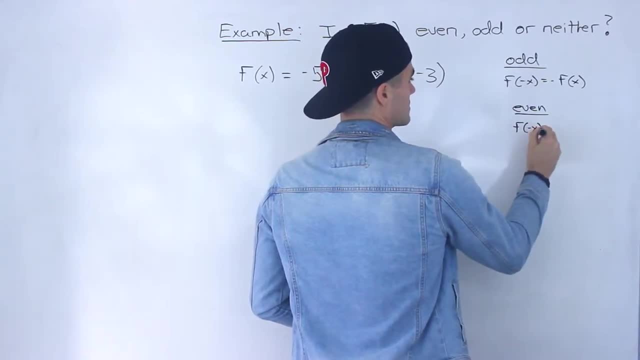 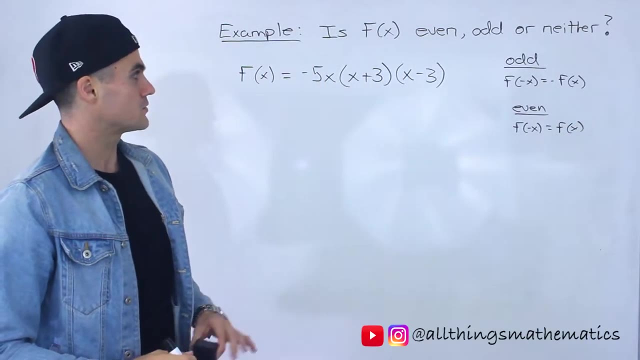 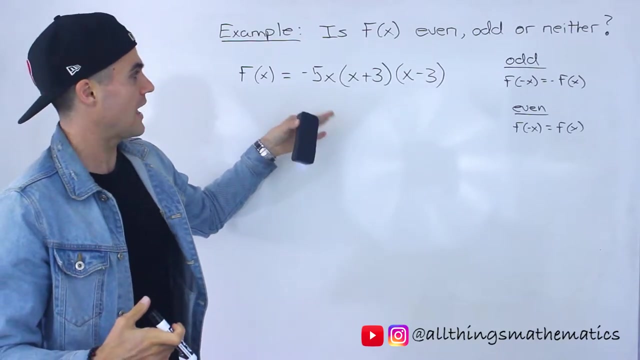 is going to be, even if f of negative x equals the original function f of x. That's how we can algebraically check this. So so far we've been dealing with polynomial functions that have been expanded. but notice, this is a polynomial function in factored form and we can expand this. the 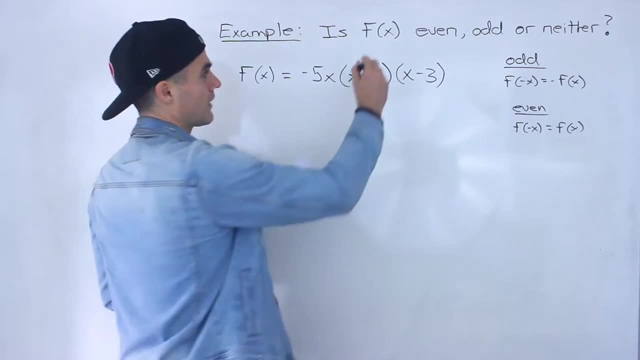 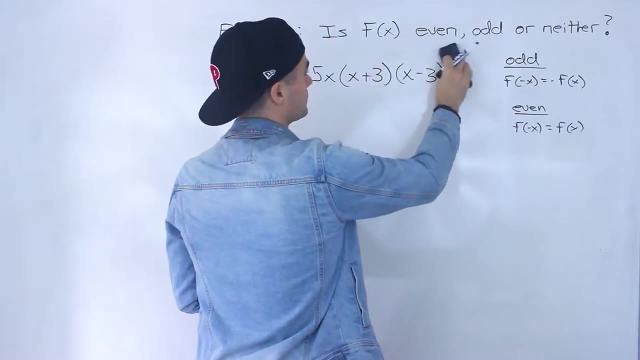 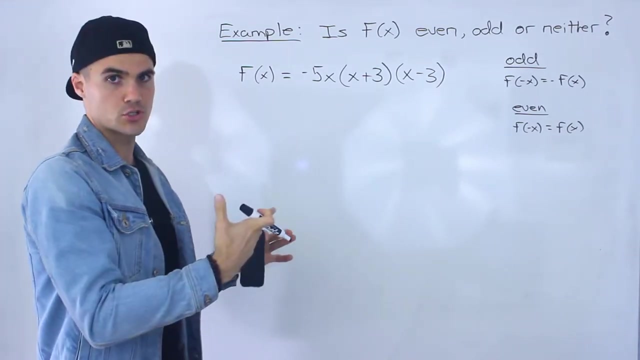 expansion on this wouldn't be too bad, actually, but what if we had an exponent two here and then an exponent three? then the expansion can get a little wild. So what we're going to be doing in the next couple of videos, starting with this one, is showing you how to find the symmetry of a. 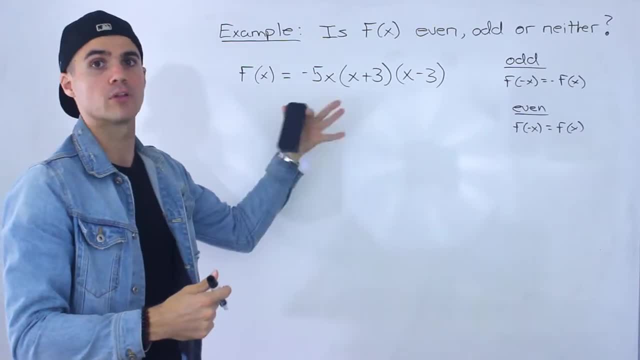 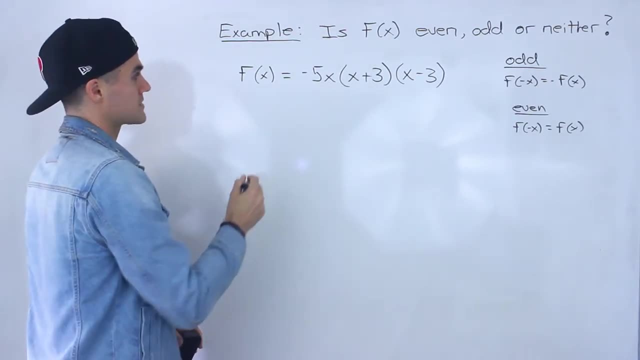 function, And it's in this factored form, and even in more complex factored form, as we'll go over in future videos, But for now let's just work with this one and let's keep it in this format. So this is f of 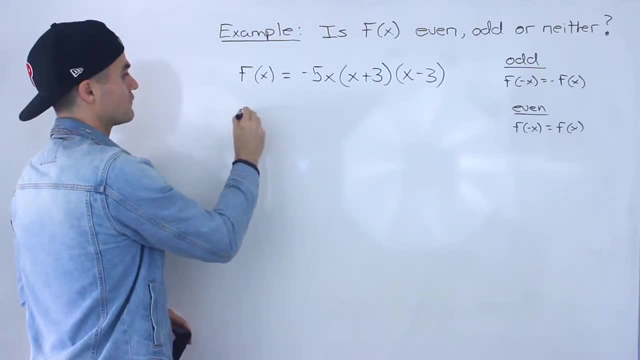 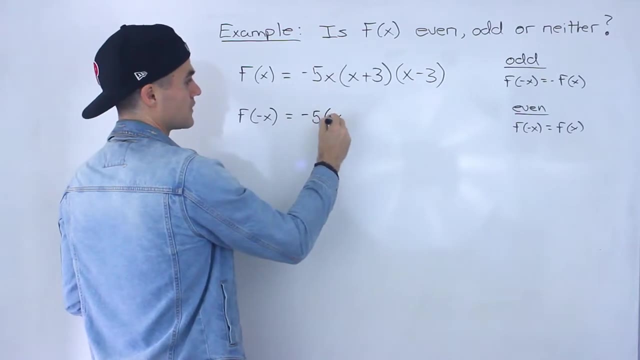 x here. So what do we got to find? We got to find out what's f of negative x first. So what we would do is we would plug in negative x for all the x values. So we have negative x over here, We'll. 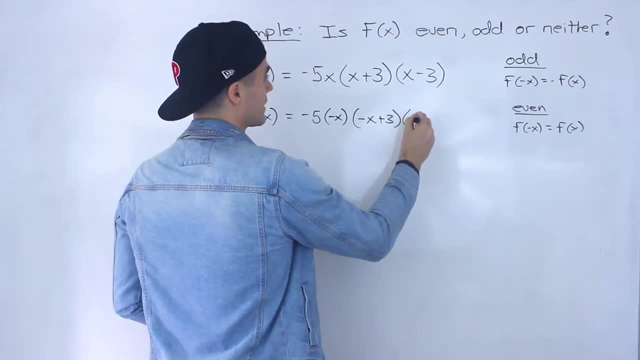 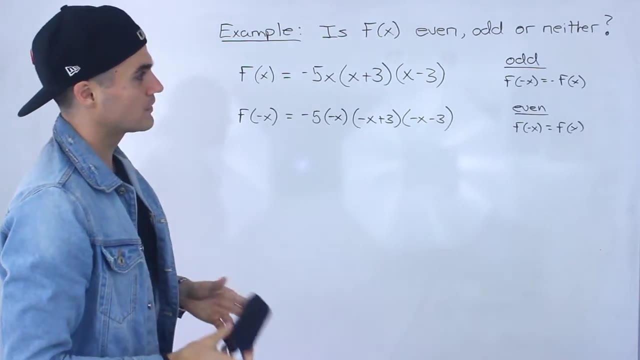 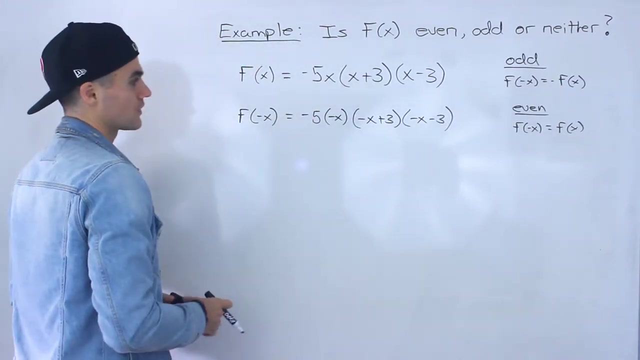 have negative x plus three here, and then we got negative x minus three. So we want to find an expression for f of negative x, and then we're going to find an expression for negative f of x and see whether any of these equalities hold here. So to simplify this, what? 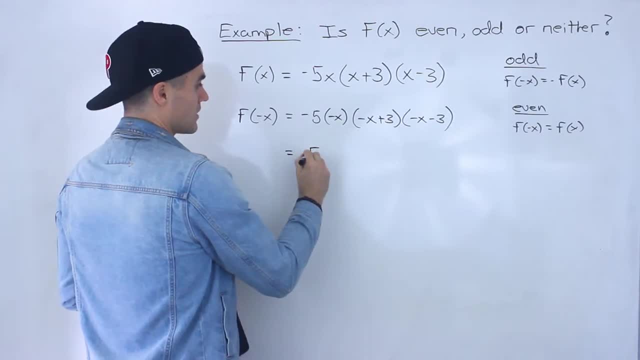 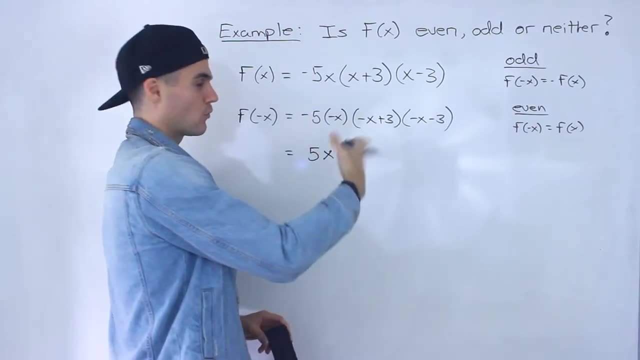 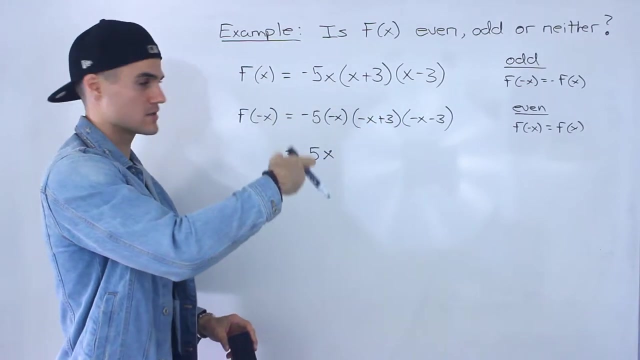 you do notice negative five times negative. x is just going to be positive five x. And what you do with these brackets here is you want to factor out a negative one from both of them because you want the same format as the original function, having a positive leading coefficient. So I'm going to 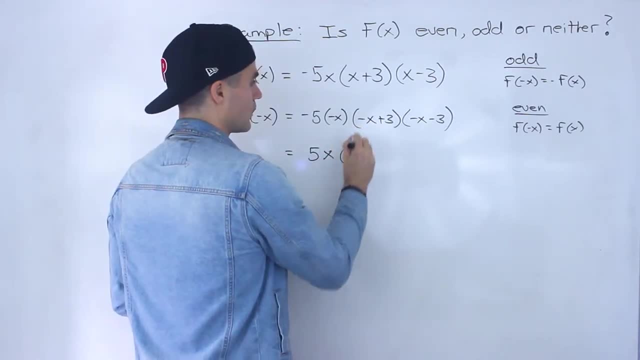 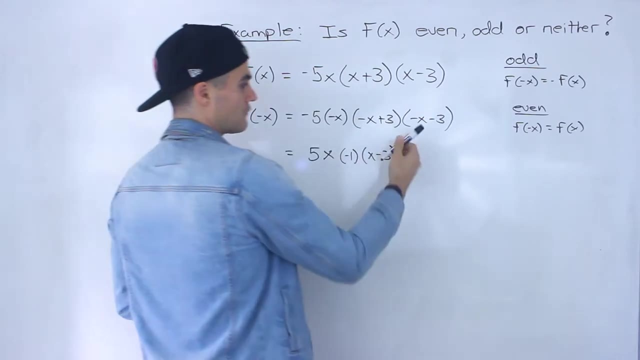 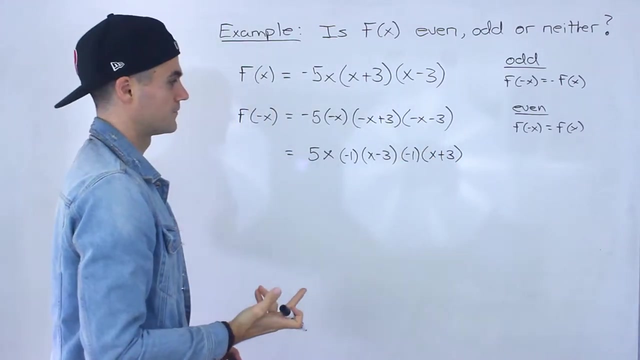 factor out a negative one here. So if I factor out a negative one from this bracket, notice, I'll end up with x minus three, Right, All the signs will change. And then if I factor out a negative one from this bracket, this would become an x plus three. All the signs will change there And now. 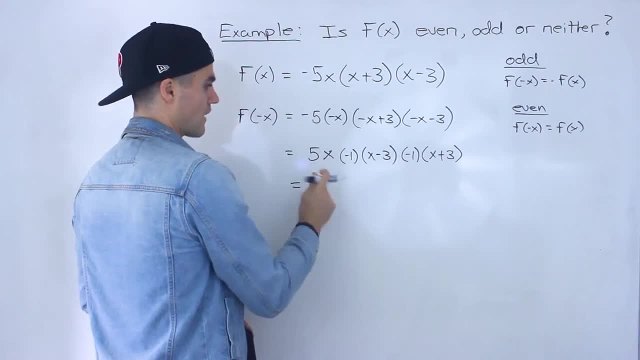 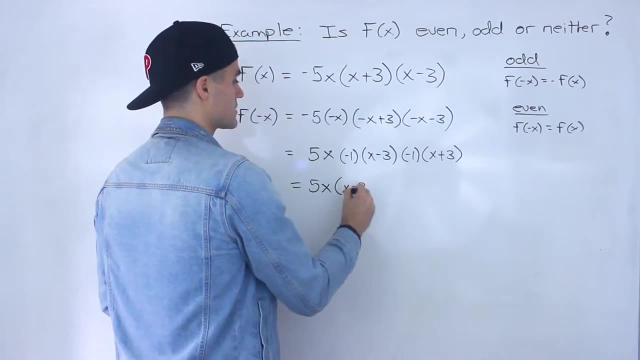 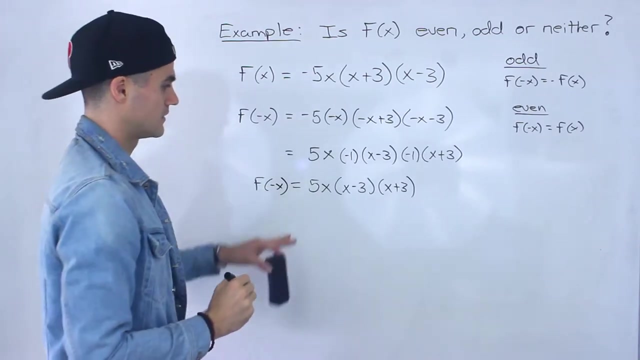 what you can do is you can multiply this: negative one, negative one, five x. So negative one times negative one, Just positive one times five x, just gives us positive five x, And then we got this x minus three, x plus three, And so that there is the simplified expression for f of negative x. 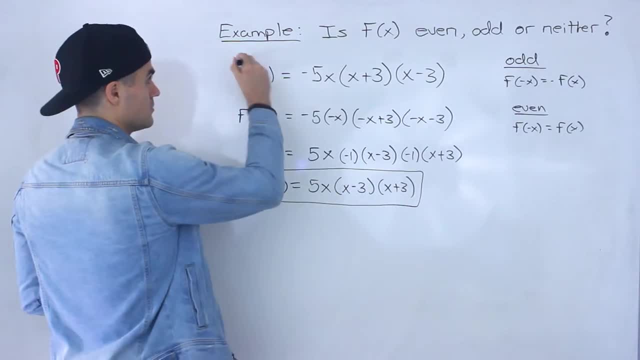 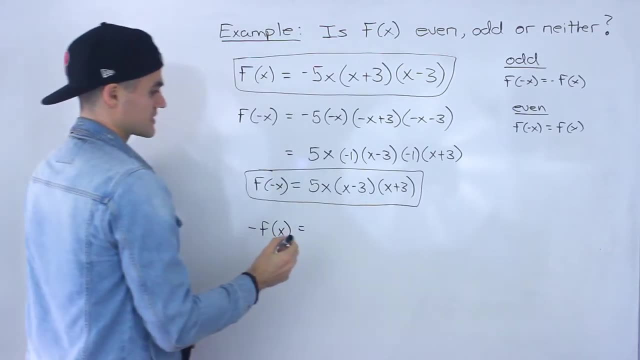 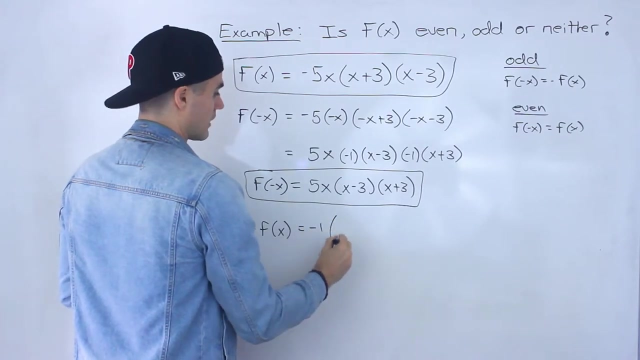 So we're going to be using this. We're also going to be using this. And then we also got to find out what's negative f of x And negative f of x in this case is very simple: We just multiply this whole thing by negative one, So we would put a negative one in front and then just rewrite. 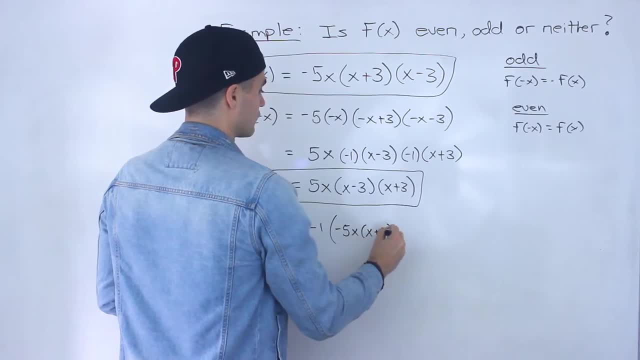 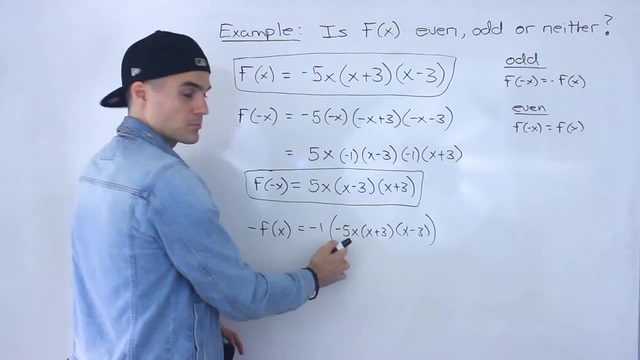 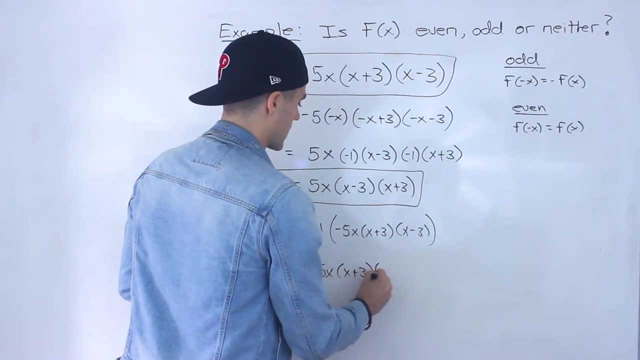 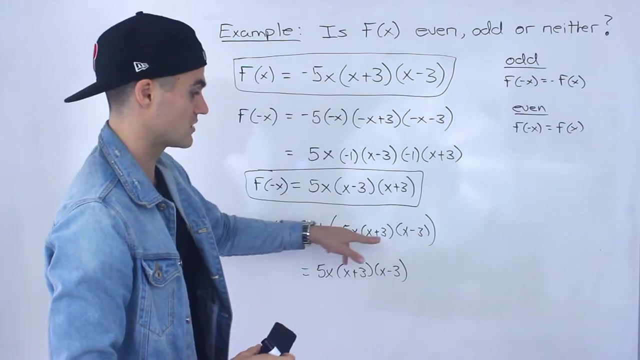 that original function And all you do here is take that negative one and multiply it by this first expression, So you would end up with positive five x x plus three x minus three. Now be careful, this negative one you don't distribute quote unquote to this expression and 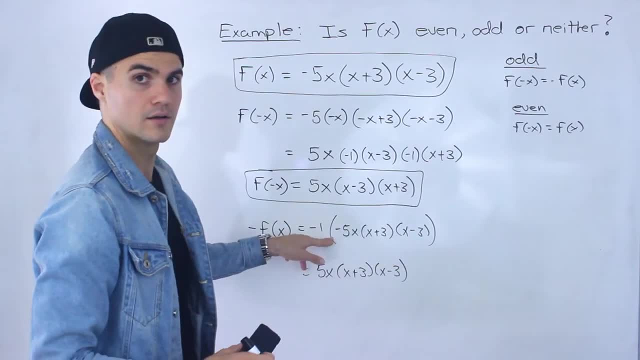 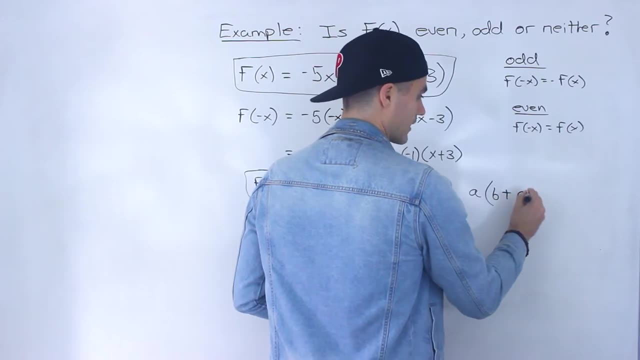 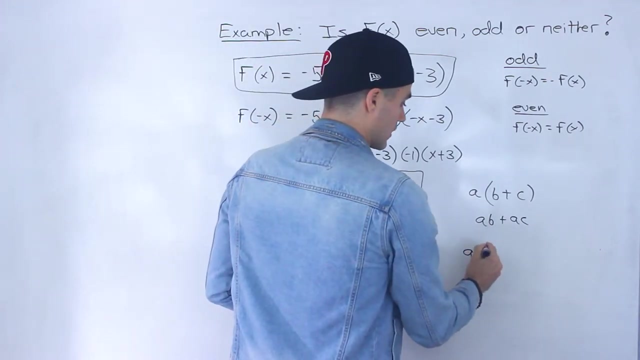 this expression and then this expression, because they're all multiplying. Okay, So just to do a quick little review of fundamentals: If you got something in front and you're adding expressions, then you can distribute. But if you got something here and you're multiplying expressions in the 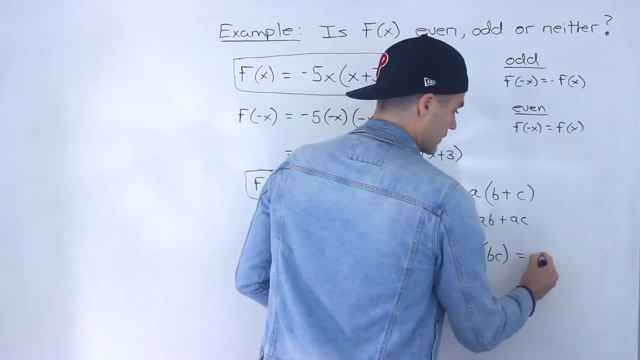 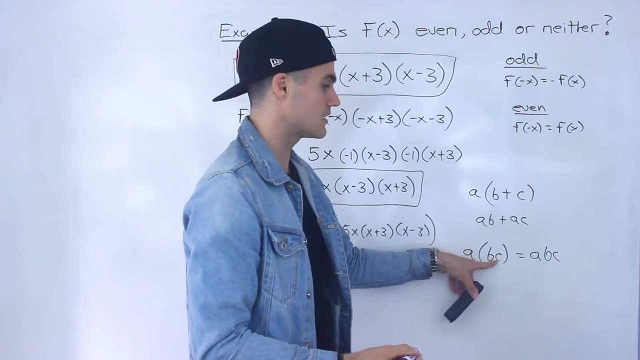 bracket, like we're doing here, then you just multiply everything You don't distribute. You don't take this a and multiply it by the b. Take the a and multiply it by the c. You don't take this a and multiply it by the c, You just multiply the a by both of these terms, like that. Okay, So the 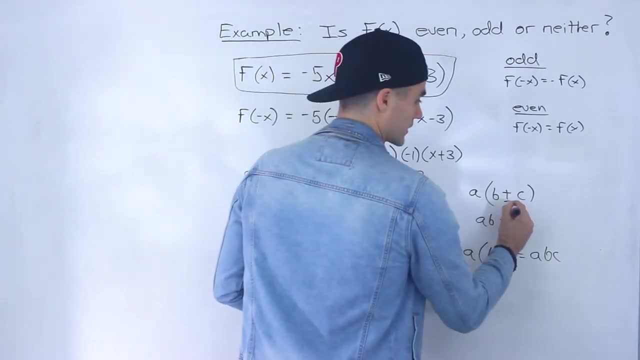 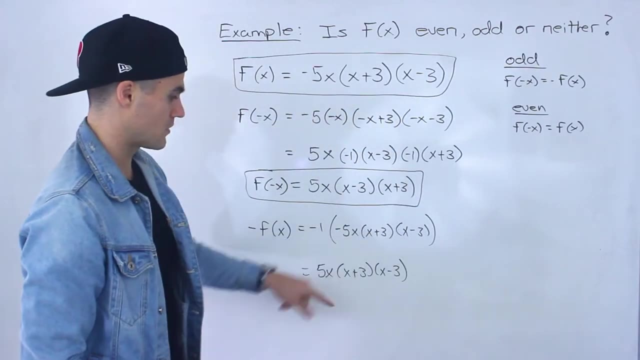 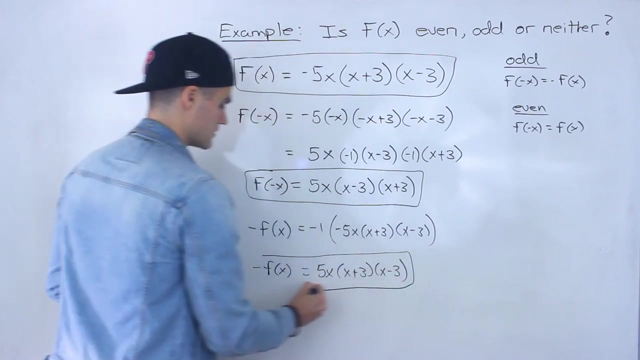 distribution. quote. unquote happens when you're adding or subtracting. This could be subtracted as well, Right? So just be careful with that. So this negative one, we're just multiplying by that first term, And so this is the expression for negative f of x. And so what you do now is you: 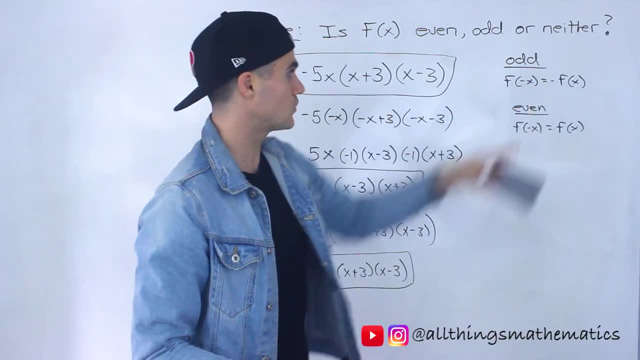 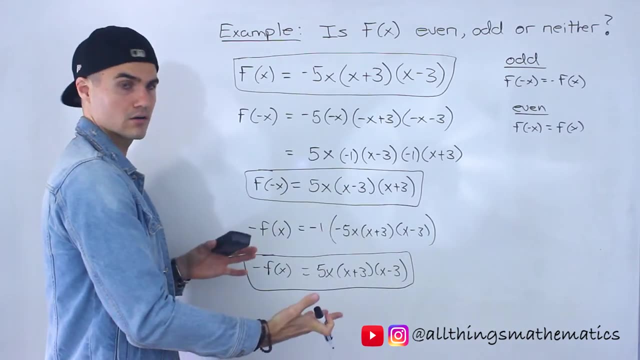 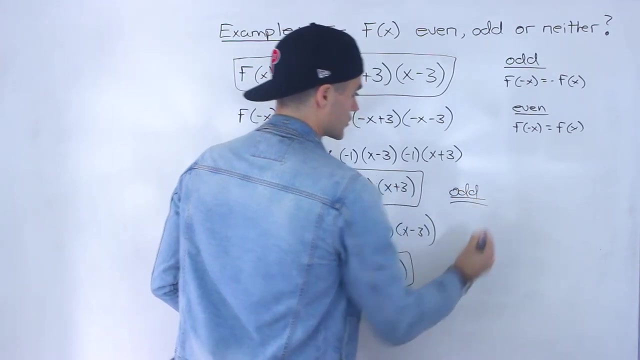 just check: does f of negative x equal Negative f of x? Well, notice f of negative x is this and negative f of x is that, and notice that they are indeed the same thing in this case. So the answer to this question is that the function. 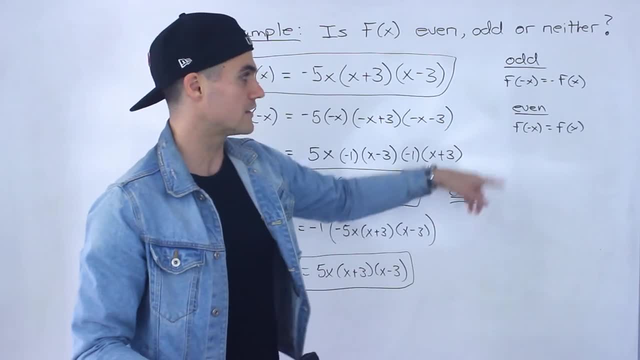 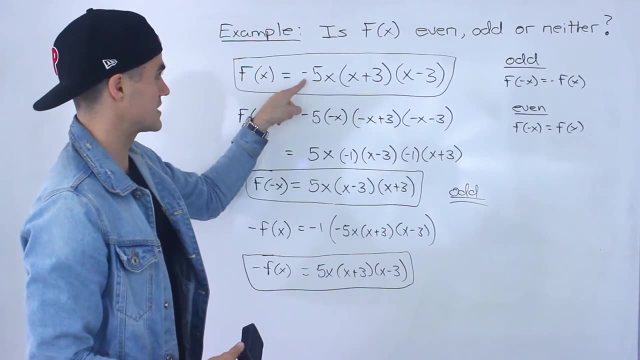 is odd. Now we could check. if it's odd, then it shouldn't be. even So, notice f of negative x, this expression, and then what's f of x? It's this, Now, they're almost the same. The factors x plus three, x minus three are the same. So they're almost the same. So they're almost the same.